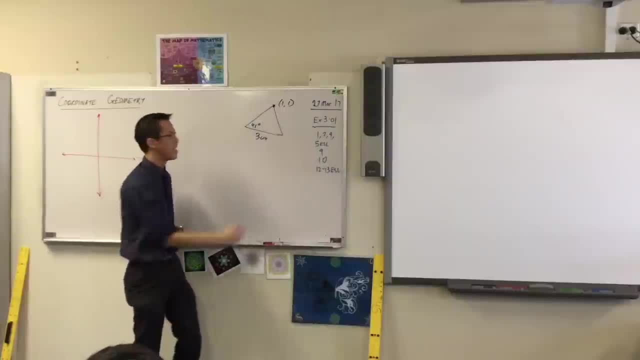 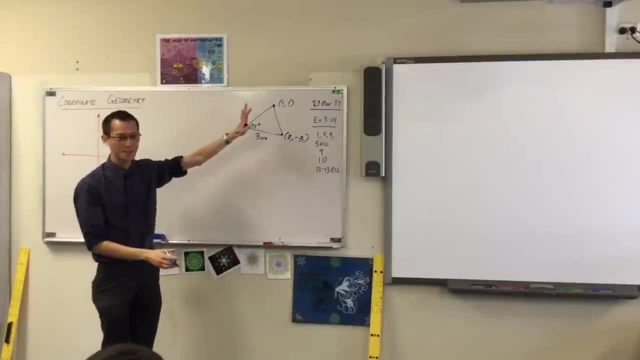 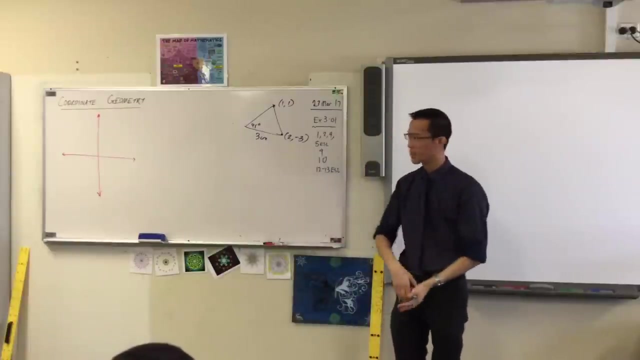 you where exactly this point is and you can understand it in relation to another point, and you can exactly see where it is in space. what that does is it unites equations which we've been dealing with earlier today, which we've been dealing with for years, equations together with shapes, now that's. 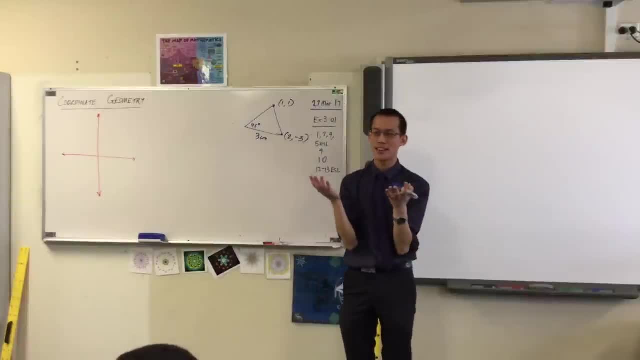 really weird. that's a little bit like: can you imagine if there was like, say, you know, in Australia- I don't know how many of you follow rugby league, but you know how there's the state of origin every year. right, is this as well? first Queensland and they're like occupying completely different sort of 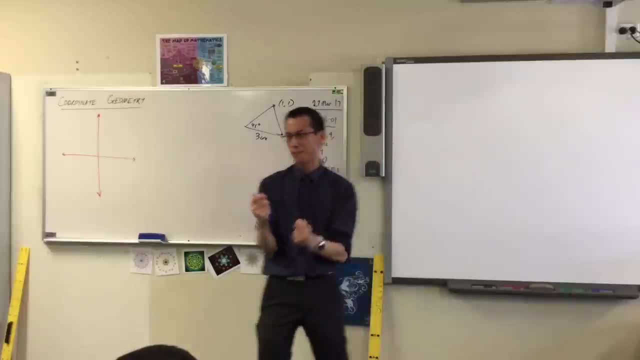 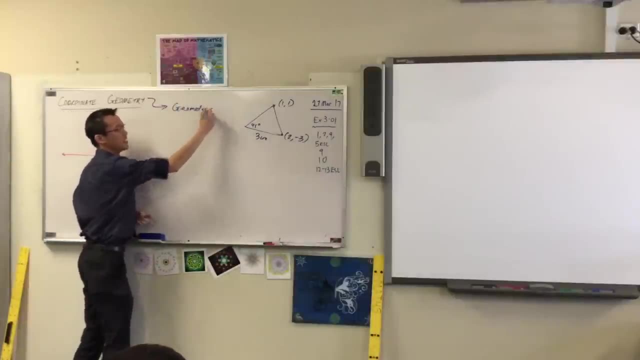 they're like: I'm against this guy and we're. we have a really bitter rivalry. people who work with geometry have a special name. they're called- I don't know if you're right this- they are called geometers, right? this is a person whose whole world and job is geometry. 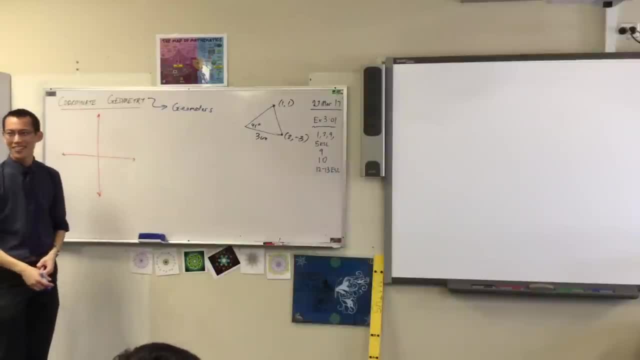 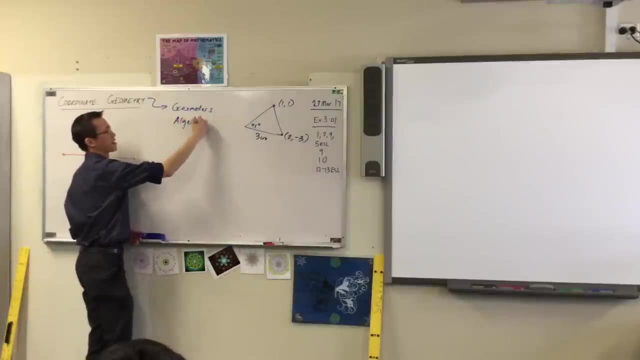 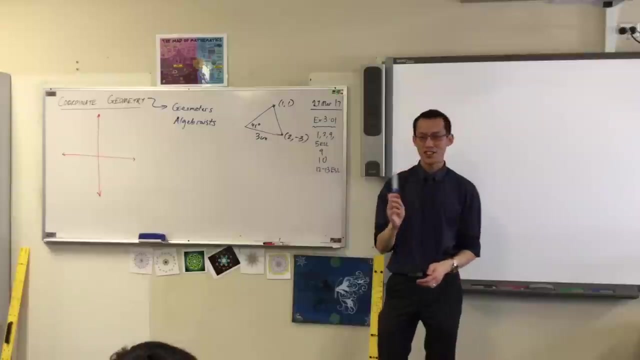 is geometry And it's a lot more fun than you might think. When you deal with equations. we have these other guys. they're often called, among other things, algebraics: algebra right Now. for centuries, shh, shh, shh, you're 10.. For centuries, these guys were like the blues. 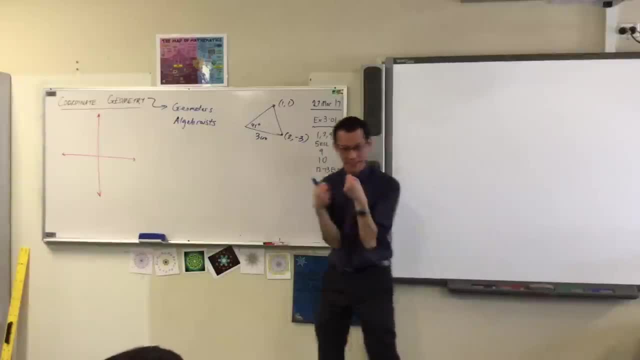 and the maroons. They're like: we have our world, you have yours and if anything, we sort of butt heads because we don't like each other. It's like you know, we love to deal with shapes and eternal sort of patterns out there and these guys like to deal with. 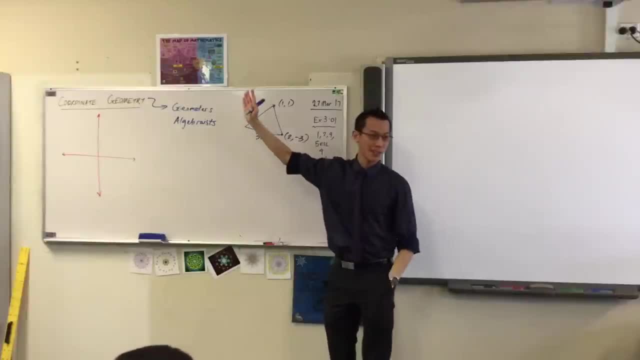 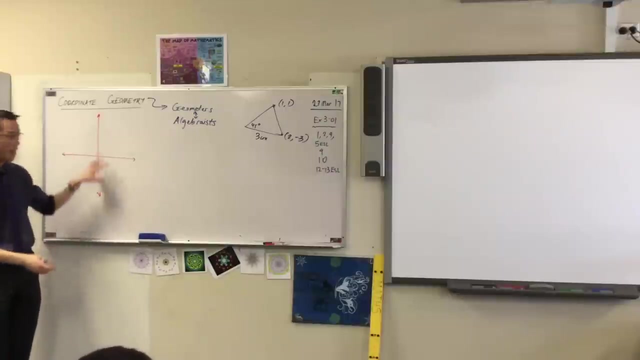 nitty-gritty details and numbers, But what coordinate geometry does is it says actually these two really importantly- complement one another. Quadrant geometry brings equations and shapes and points and lines together into one coherent whole. That's why we spend time on this, okay. So I want us to try and remember a little bit about the language. 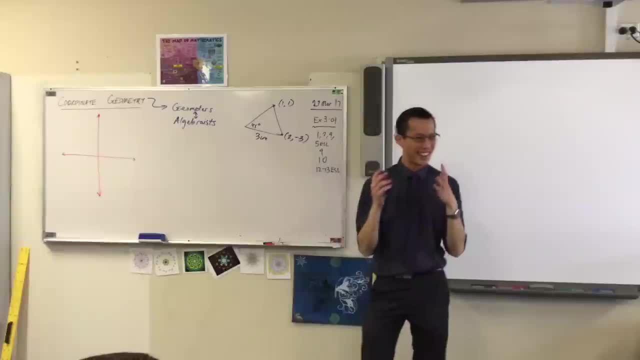 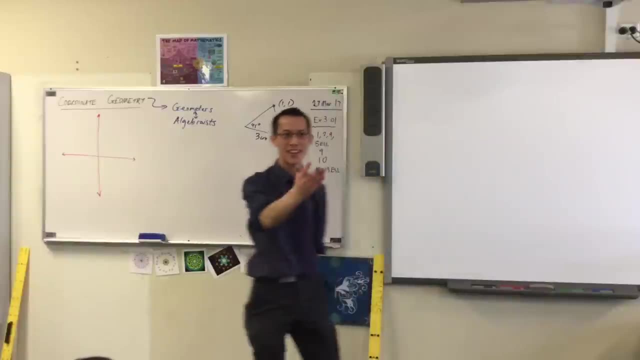 You want us to try to stick to the language of how coordinate geometry works, To go back to year seven. And this thing- And does anyone remember It- has a name. Actually, it has a French name. Does anyone remember what it is? Yeah, this is called the Cartesian plane. 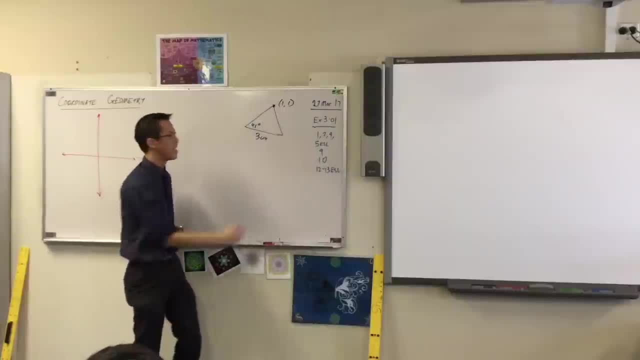 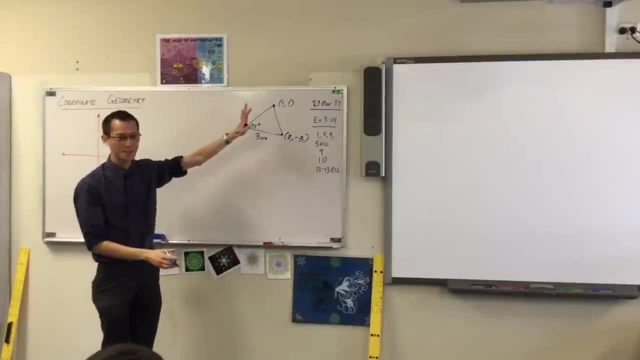 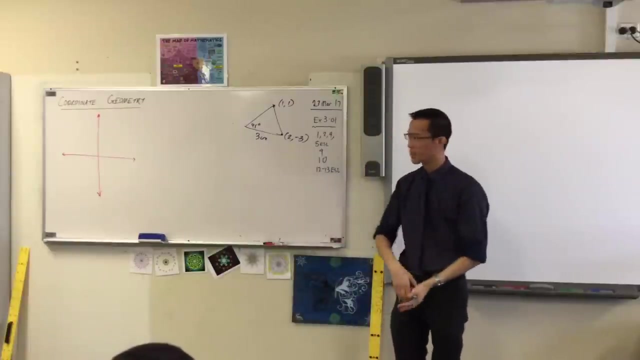 you where exactly this point is and you can understand it in relation to another point, and you can exactly see where it is in space. what that does is it unites equations which we've been dealing with earlier today, which we've been dealing with for years, equations together with shapes, now that's. 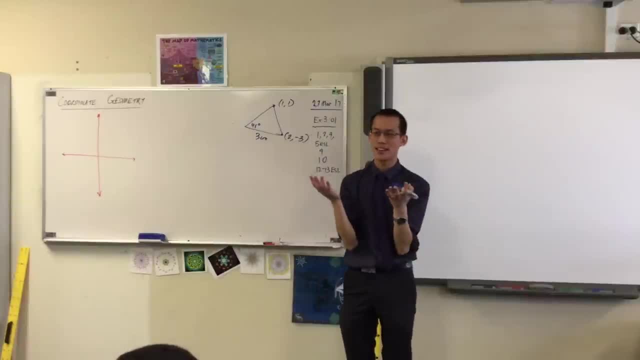 really weird. that's a little bit like: can you imagine if there was like, say, you know, in Australia- I don't know how many of you follow rugby league, but you know how there's the state of origin every year, right is this? that's Wales vs Queensland and they're like occupying completely different sort of they're. 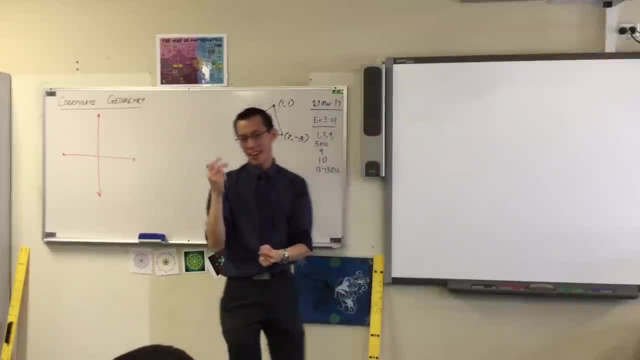 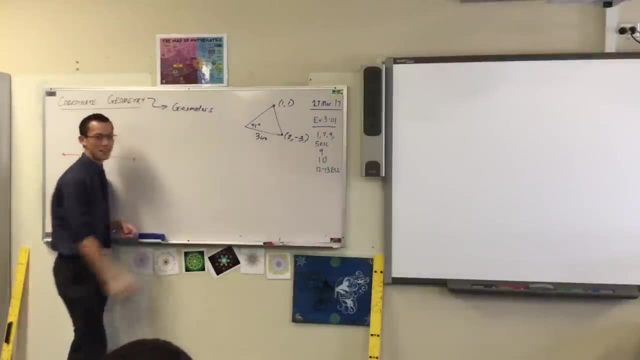 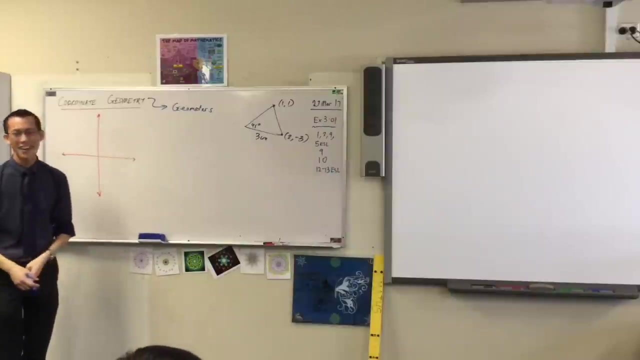 like I'm against this guy and where we have a really bitter rivalry. people who work with geometry have a special name. they're called- I don't know if you write this- they are called geometers, right? this is a person whose whole world and job is geometry, And it's a lot more fun than you might think When you deal with equations. 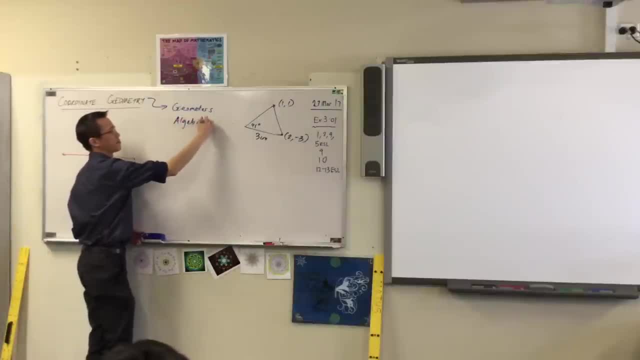 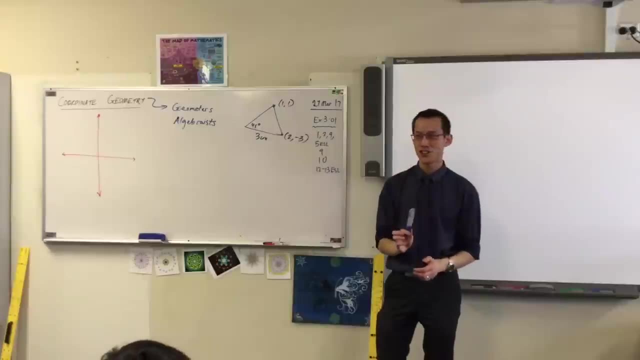 we have these other guys. they're often called, among other things, algebraics. algebra right Now. for centuries, shh, shh, shh, you're 10.. For centuries, these guys were like the blues and the maroons. They're like: we have our world, you have yours and, if anything, we. 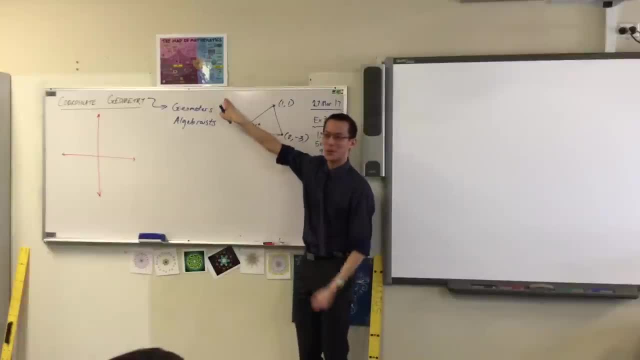 sort of butt heads because we don't like each other. It's like you know, we love to deal with shapes and eternal sort of patterns out there and these guys like to deal with nitty-gritty details and numbers. But what coordinate geometry does, is it says actually. 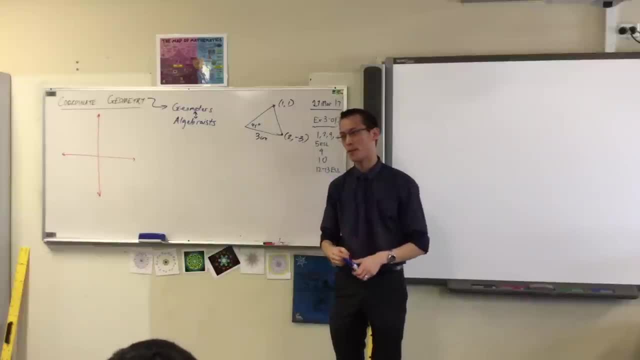 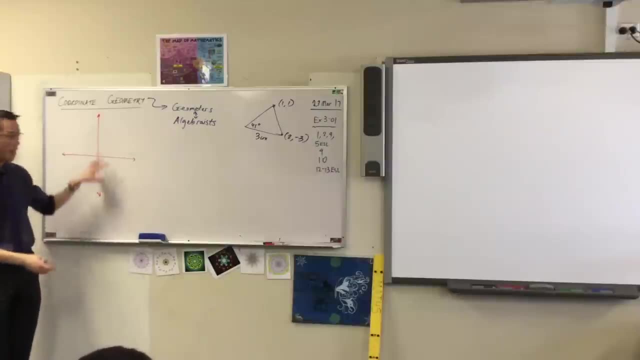 these two really importantly complement one another. Quadrant geometry brings equations and shapes and points and lines together into one coherent whole. That's why we spend time on this, okay, So I want us to try and remember a little bit about the language. 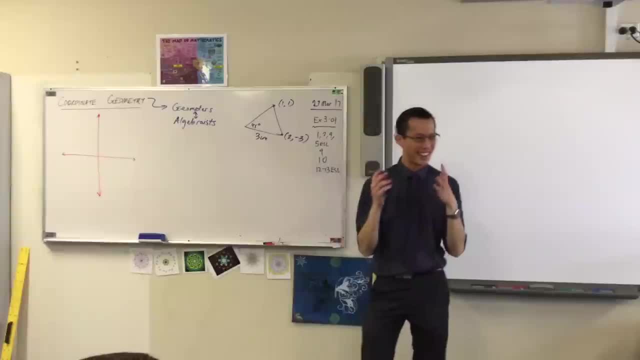 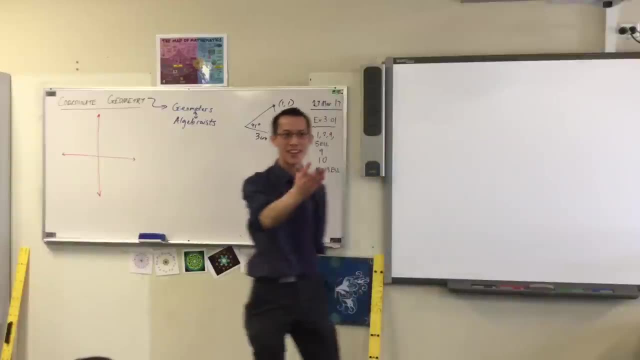 The language of how coordinate geometry works, To go back to year seven and this thing: Does anyone remember? It has a name. Actually, it has a French name. Does anyone remember what it is? Yeah, This is called the Cartesian plane. Can you off on the side here? can? 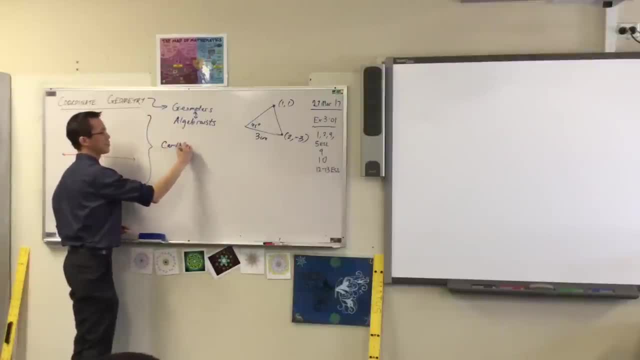 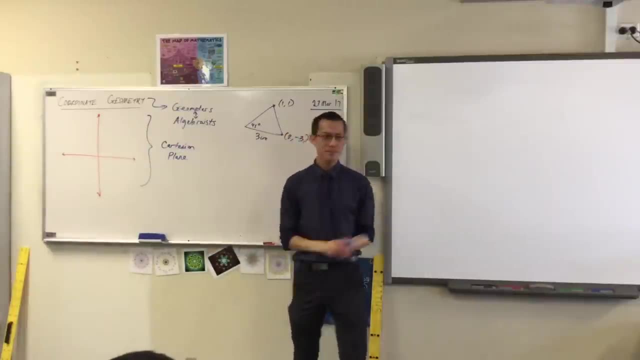 Can you off on the side here. Can you label this the Cartesian plane, The plane not to be confused with a thing that flies through the air? In this context, planes are very, most of the time are in order, So they're on a large scale in the same place in a. 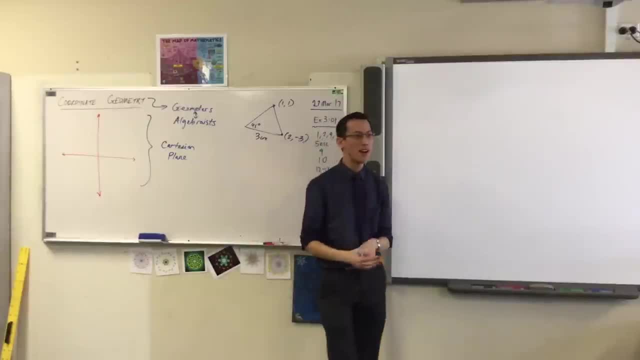 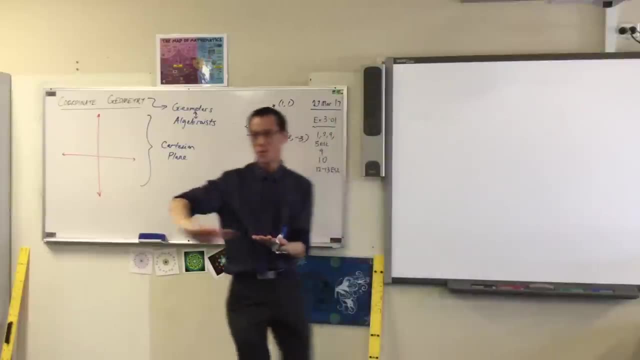 Plain just means something flat, Okay. so if you guys remember, when you're doing woodwork and you're trying to make something flat, you use a Plain Plain because you're trying to smooth it all out and chisel off whatever wood is making it bumpy, okay? 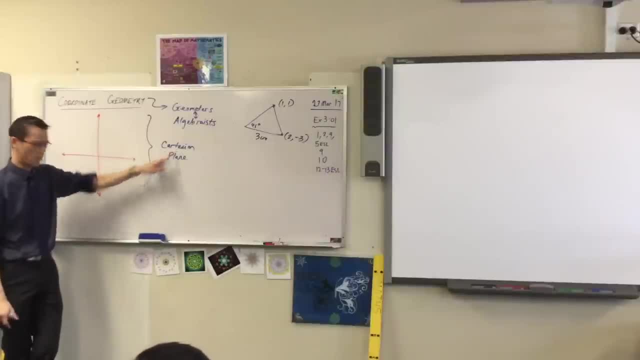 That just means a flat surface. Does anyone know where this comes from? Anyone know where Cartesian, where that comes from? Cart and Persian, So it's French. it's actually named after a guy, the guy who pioneered working on this. 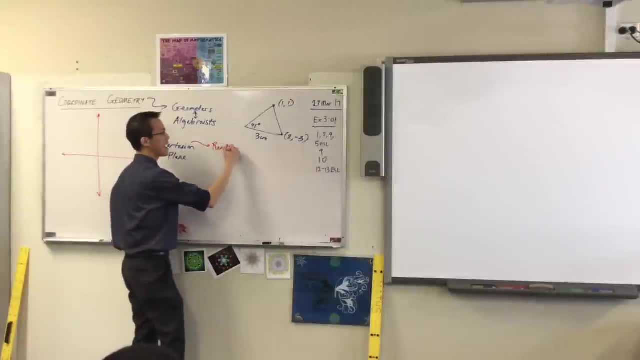 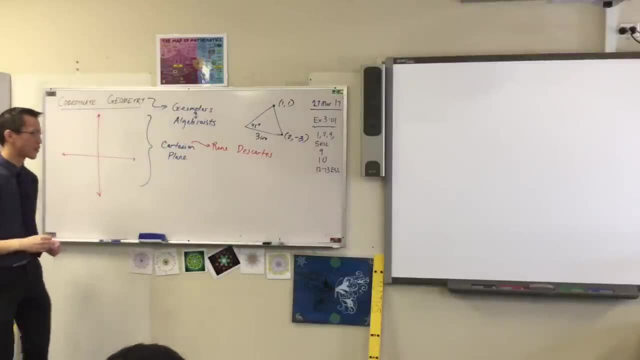 and his name is. you should write this down: his name is René Descartes. Don't pronounce that, like I used to when I was in Year 10.. Don't pronounce that, Descartes. That's not no, it's French, okay. 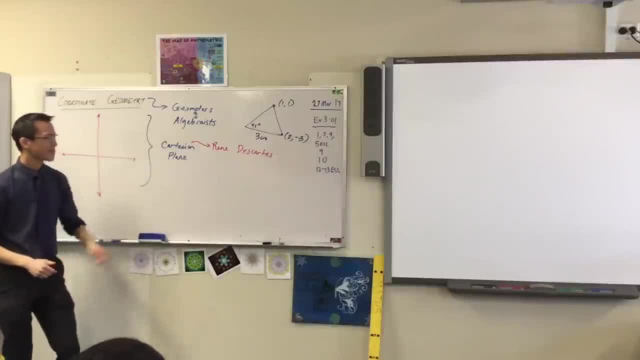 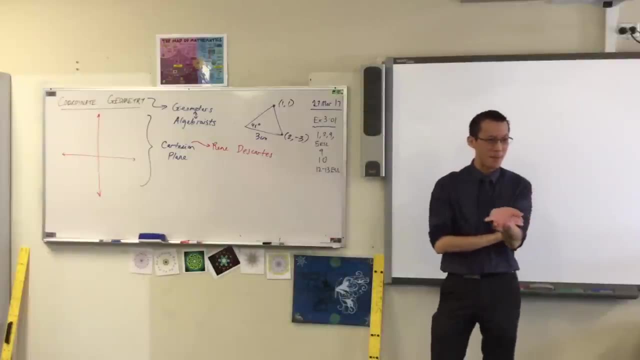 So René Descartes- He's famous for the quote, if you've heard it before, I think. therefore I am- He wasn't just a mathematician, he was into philosophy and all kinds of things. He did some cool stuff. 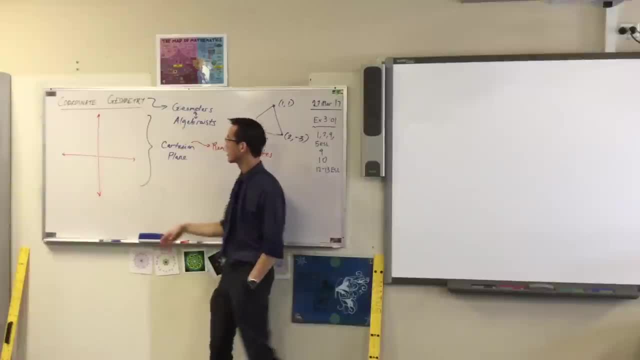 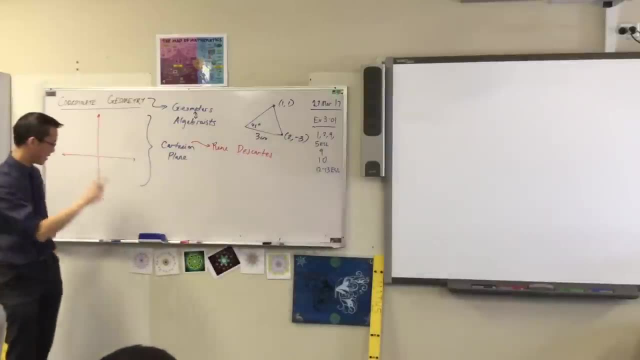 But he was the one who really, among the many people who were trying to understand how to use this thing, he was the one after whom it was named, because he did the most work with it. Now, on the Cartesian Plain, there is one point that is more important. 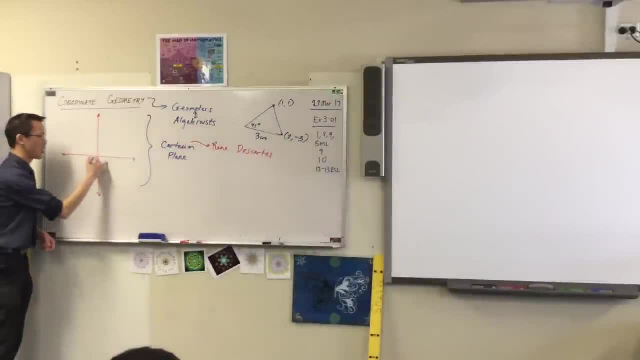 than all the rest of the points. It's the origin. So because it's important to get its own special name, and we label it O for origin right there in the centre, in order to describe where you are on the Cartesian Plain. 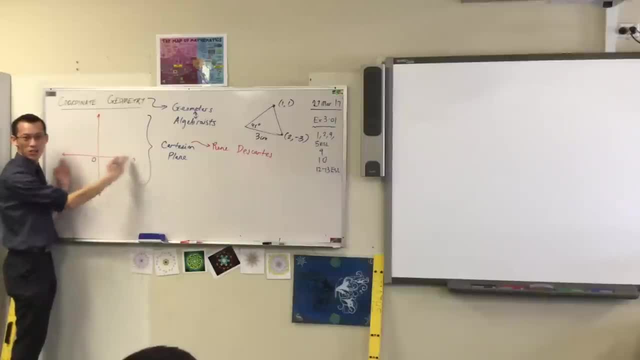 you only need two numbers. You need to know where you are horizontally and where you are vertically. So we give these two things. rather than saying horizontally and vertically, which are really long words with lots of syllables, we give them short names, namely: 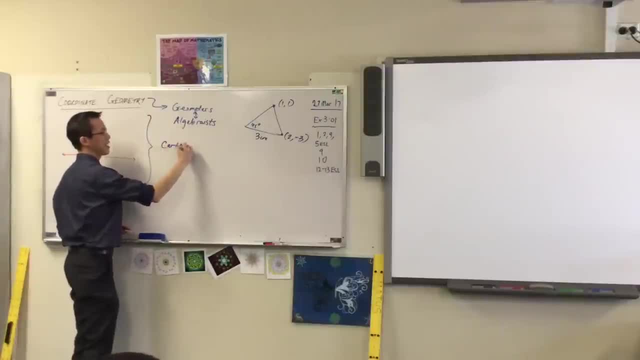 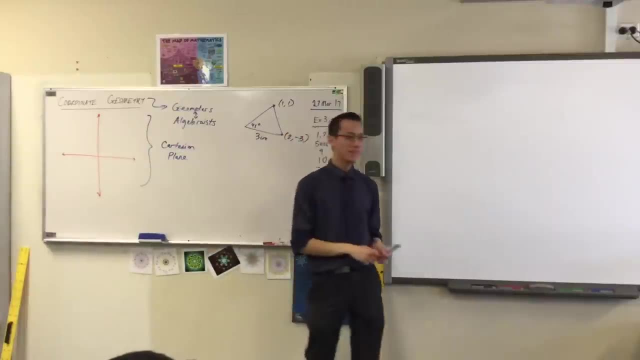 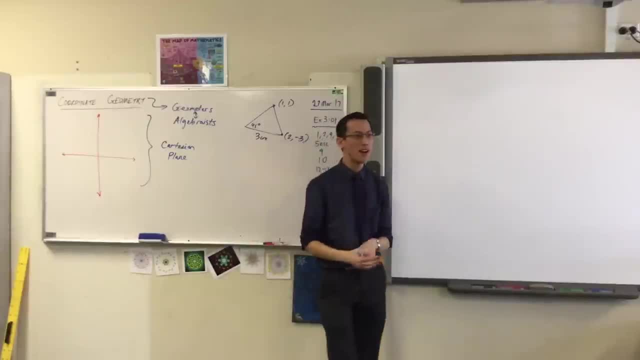 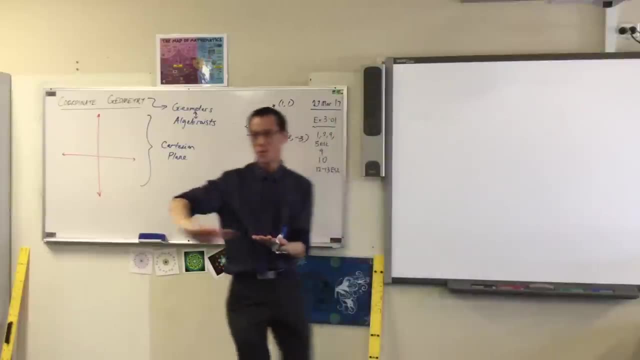 Plain just means something flat. Okay, so, if you guys remember, when you're doing woodwork and you're trying to make something flat, you use a Plain Plain because you're trying to smooth it all out and chisel off whatever wood is making it bumpy. 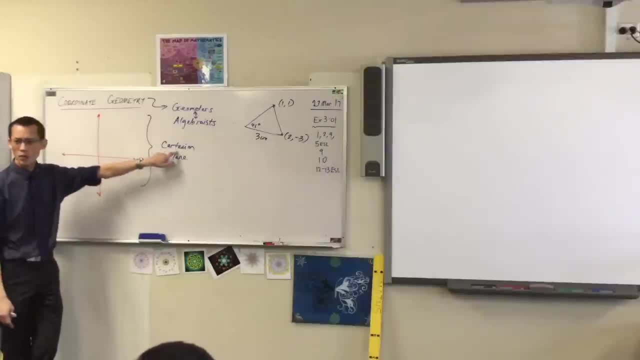 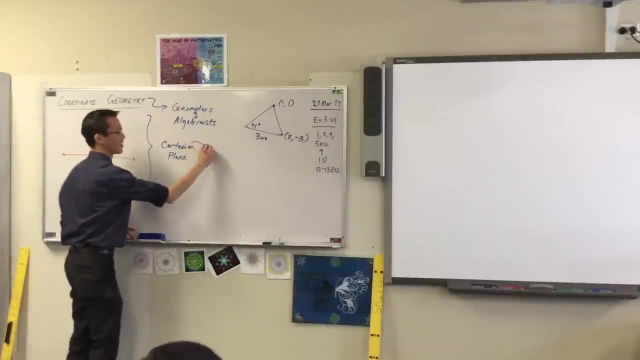 Okay, That just means a flat surface. Does anyone know where this comes from? Anyone know where Cartesian, where that comes from? So, Persian cart, It's French. it's actually named after a guy, the guy who pioneered working on this. 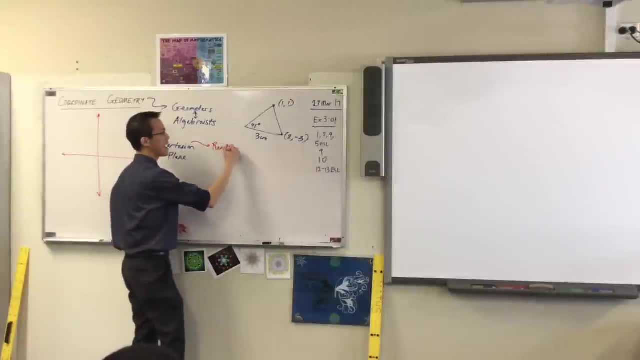 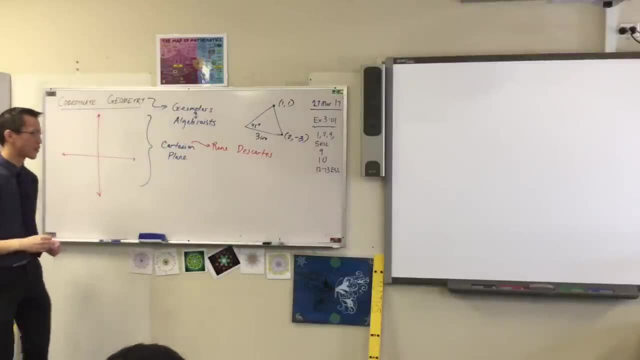 and his name is. you should write this down: his name is René Descartes. Don't pronounce that, like I used to when I was in Year 10.. Don't pronounce that, Descartes. No, it's French, okay. 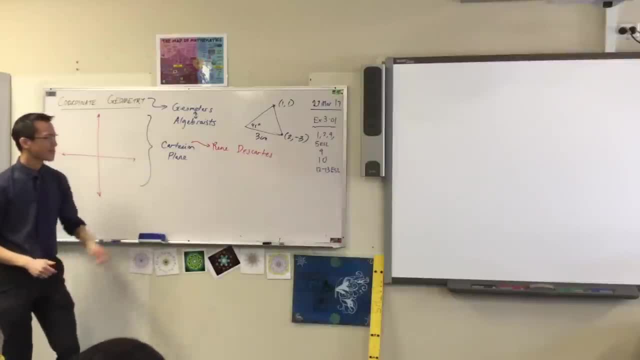 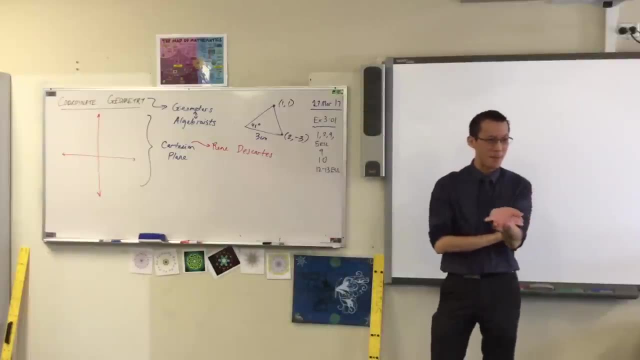 So René Descartes- He's famous for the quote, if you've heard it before, I think. therefore, I am. He wasn't just a mathematician, he was into philosophy and all kinds of cool stuff, But he was the one who really 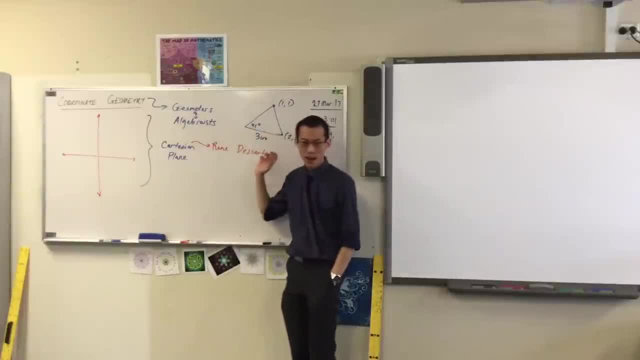 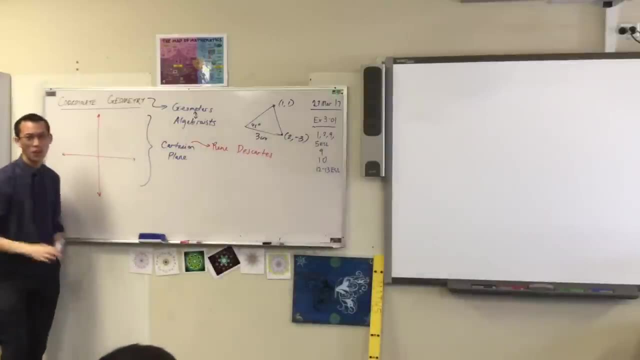 among the many people who were trying to understand how to use this thing, he was the one after whom it was named, because he did the most work with it. Now, on the Cartesian Plain, there is one point that is more important than all the rest of the points. 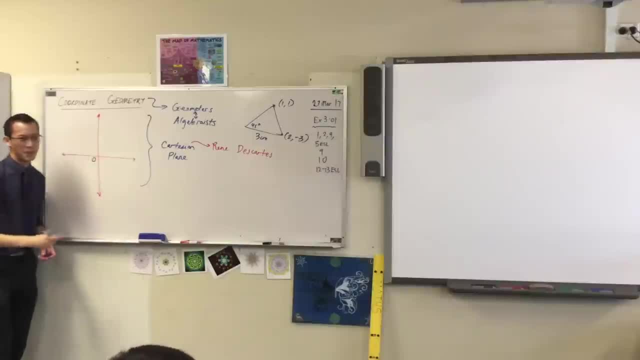 Does anyone know what it is? It's the origin. So because it's important, it gets its own special name and we label it O for origin, right there in the centre, In order to describe where you are on the Cartesian Plain. 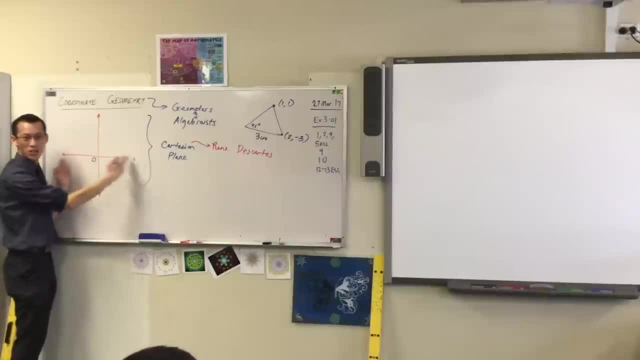 you only need two numbers. You need to know where you are horizontally and where you are vertically right. So we give these two things. rather than saying horizontally and vertically, which are really long words with lots of syllables, we give them short names, namely: 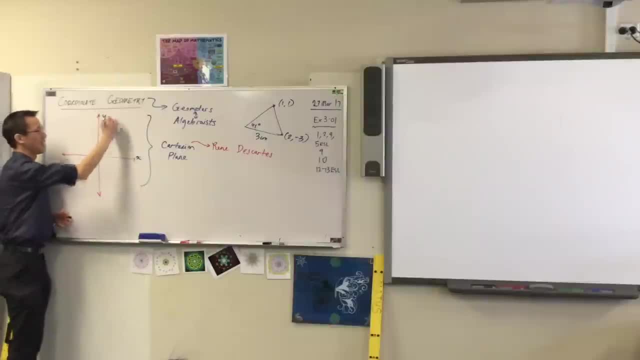 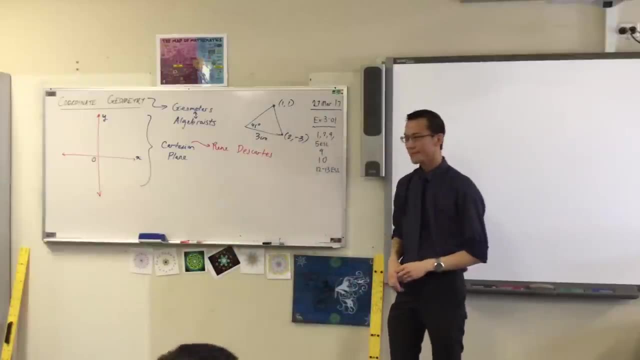 x and y. So you've got an x-axis, that's the horizontal line, you've got a y-axis, the vertical line. and if you were to not just do a plane, which is flat, but if you wanted a space with three dimensions, 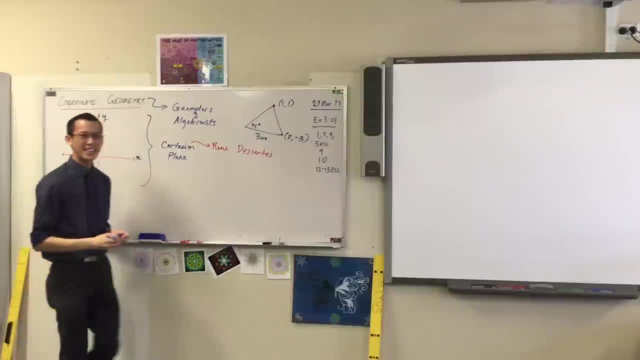 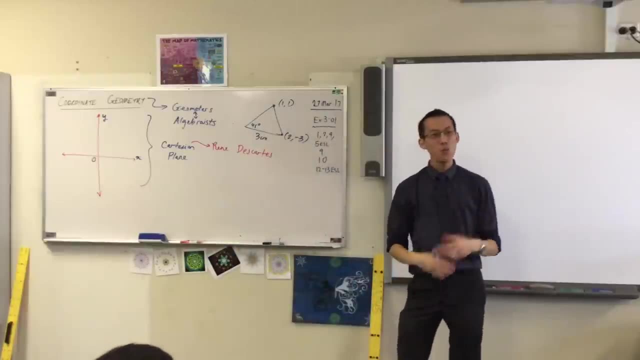 x and y. So you've got an x-axis, that's the horizontal line, You've got a y-axis, the vertical line. And if you were to not just do a plane which is flat, but if you wanted a space with three dimensions, 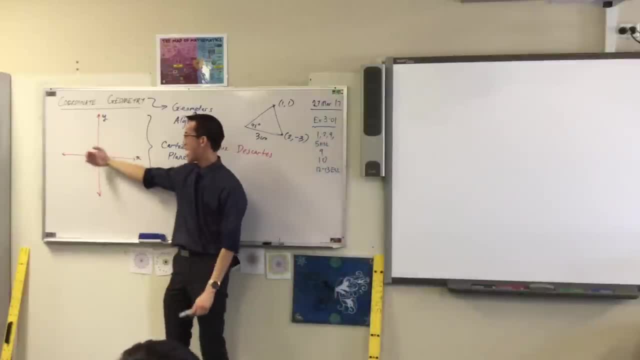 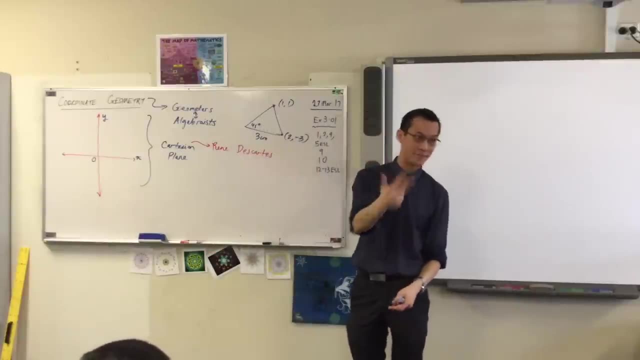 like the one we live in: x and y. you'd also have z, which is sort of coming out of the board, And then you can describe 3D space. It's 3D because there's an x and a y and a z. 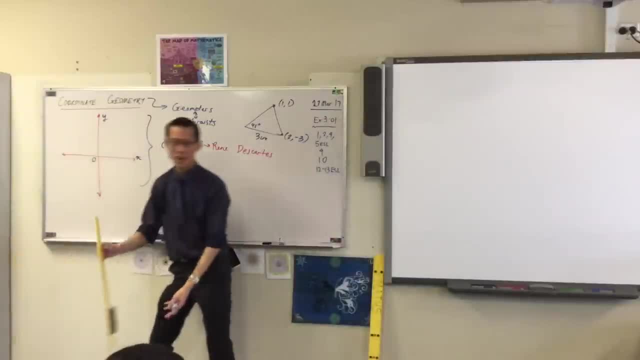 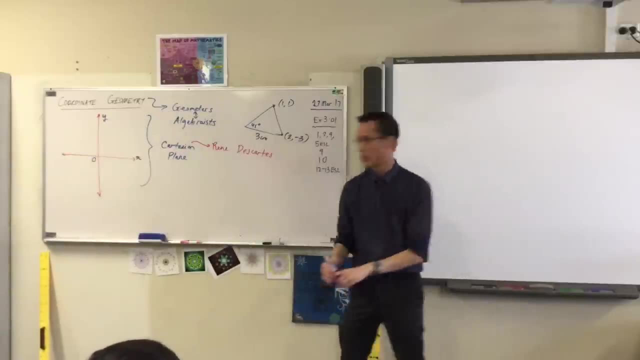 But this is 2D. Just imagine have another third axis just coming out of the board like that. except you can't do it because that's my board. Alright, let's put some points on here. So what I want you to note is: 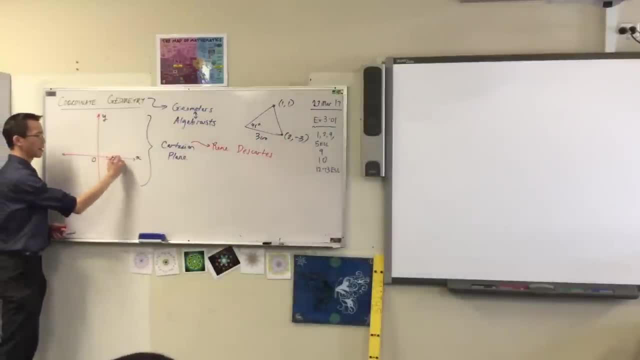 we're going to have a scale on here, So I'm going to put a few markings which I'd like you to also include. I'm going to read mostly, so this is really easy for you, So I'm going to put some markings here. 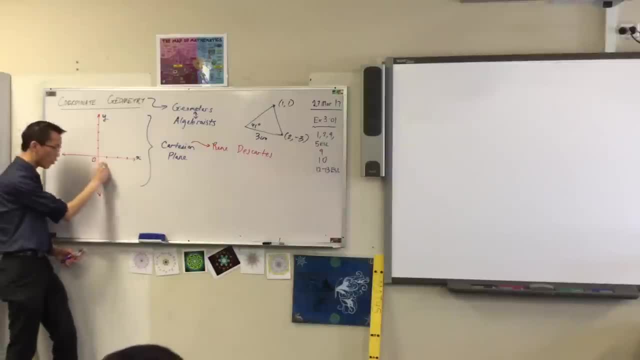 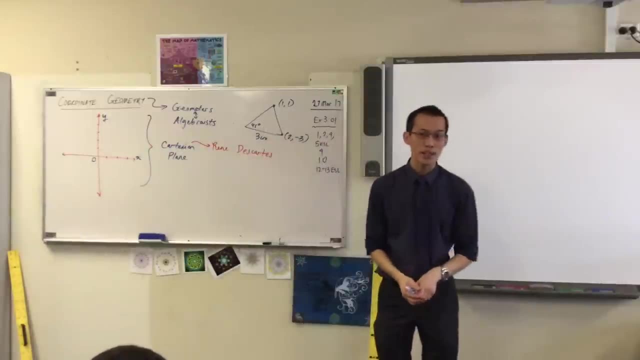 but I'm going to say to you right now: please do not mark in all of the numbers on the Cartesian plane, For two reasons. Number one: it will take you forever and almost certainly you don't need all of the numbers there. 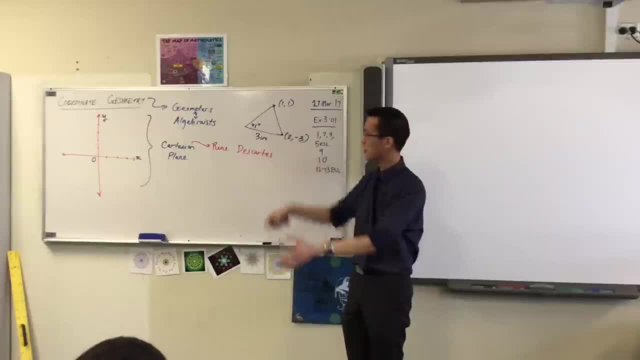 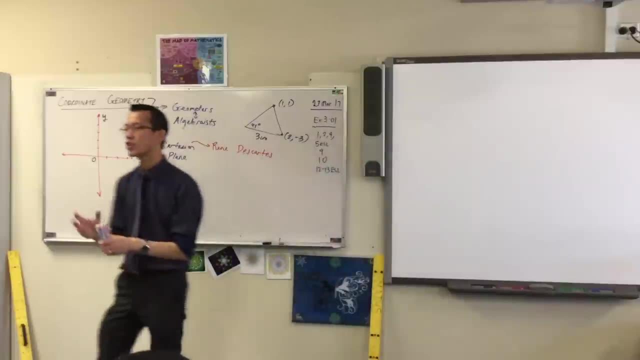 You usually only need a handful. Secondly, not only is it very time consuming just to write 1,, 2,, 3, and it becomes difficult to see all the rest of the stuff which is more important. So we're just going to label a few important bits. 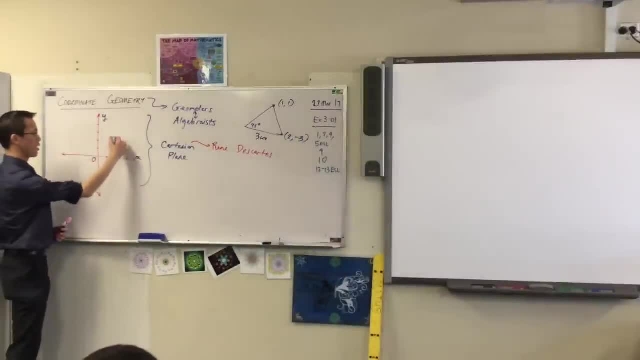 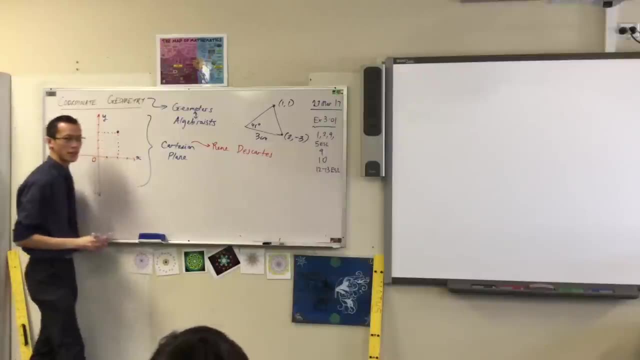 Let's pick a point. So, for instance, if I picked a point, say: there, I'm going to draw that in which is in line with this, Someone raise their hand and describe. how would we describe the coordinates of that point I drew up there? 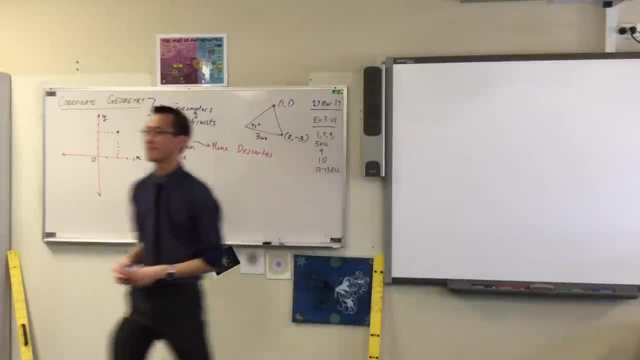 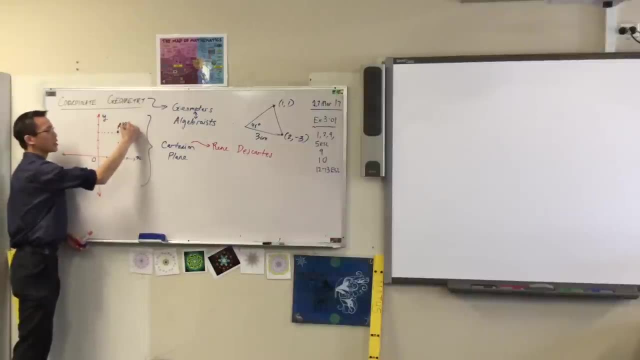 Any take? Yeah, Helen, 2, 3.. Yeah, so I'm going to label this. Let's call this guy A, And its coordinates do look like 2, 3. Because, as you can see, you've gone across 2 units. 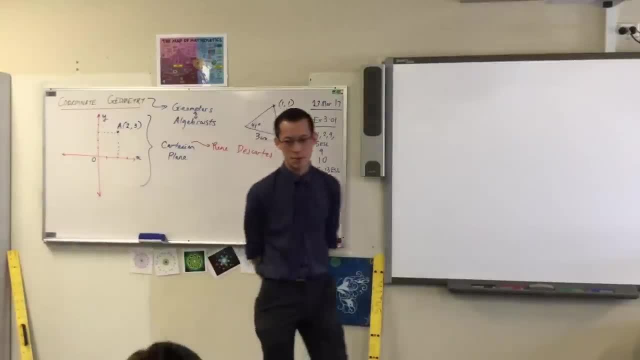 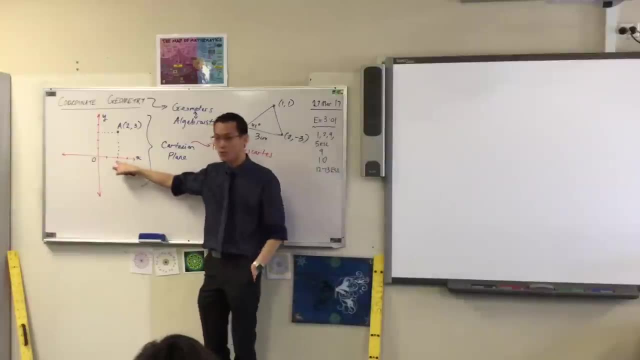 then you've gone over 3.. I will point out- I don't know if you started to draw numbers, because I was telling you not to, but I did not draw numbers, so that might not be 2, 3. It could be like 200, 300. 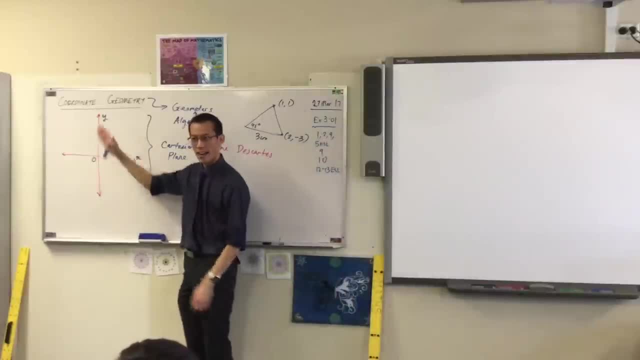 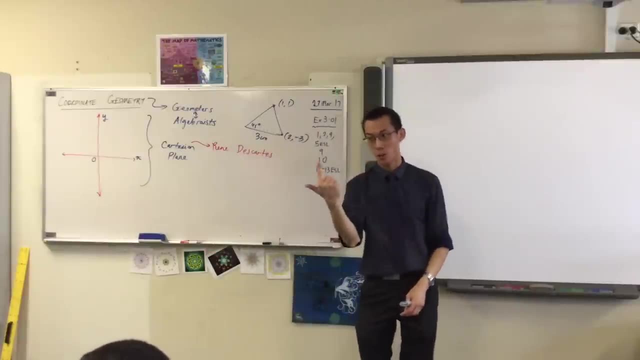 like the one we live in. then you wouldn't just have x and y, you'd also have z, which is sort of coming out of the board, and then you can describe 3D space. It's 3D because there's an x and a y and a z. 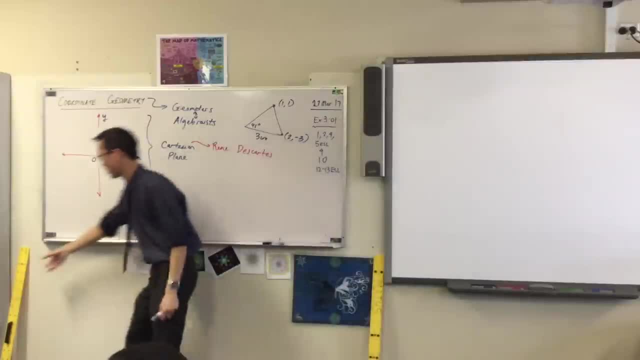 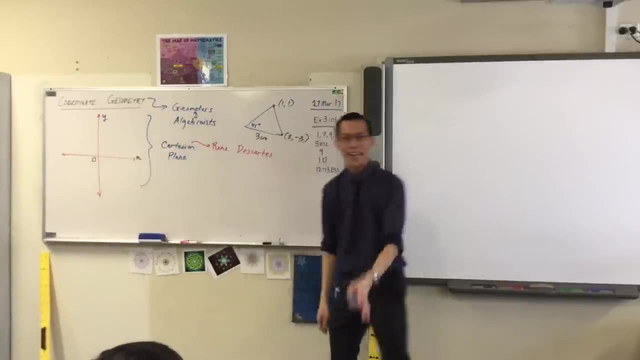 But this is 2D. okay, Yeah, just imagine just have another third axis just coming out of the board like that. except you can't do it because that's my board. Alright, let's put some points on here. So what I want you to note is: 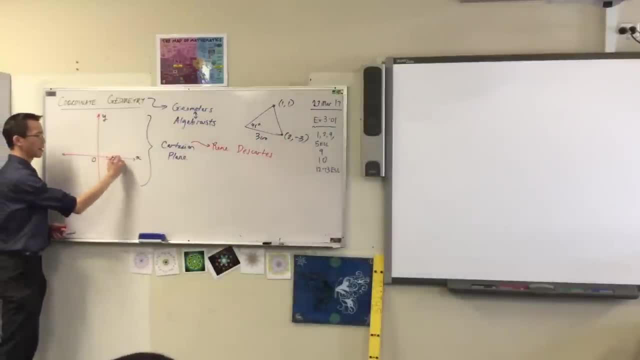 we're going to have a scale on here, so I'm going to put a few markings which I'd like you to also include. You've got a grid mostly, so this is really easy for you, So I'm going to put some markings here. 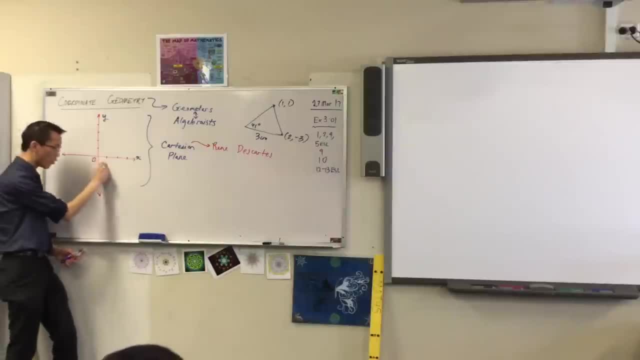 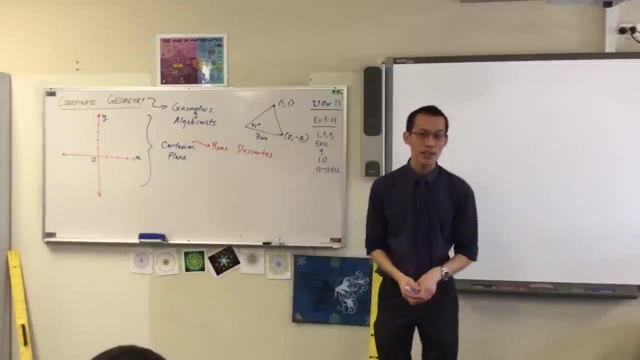 but I'm going to say to you right now: please do not mark in all of the numbers on the Cartesian plane, okay, For two reasons. Number one: it will take you forever and almost certainly you don't need all of the numbers there. 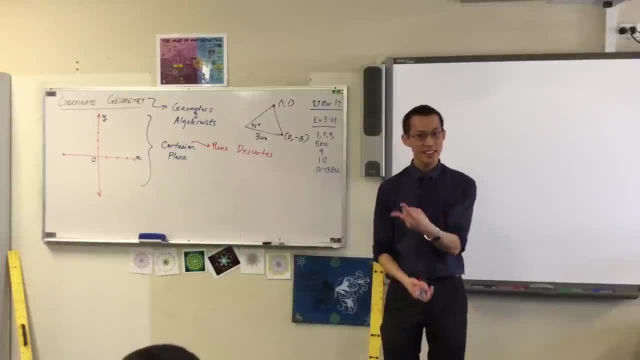 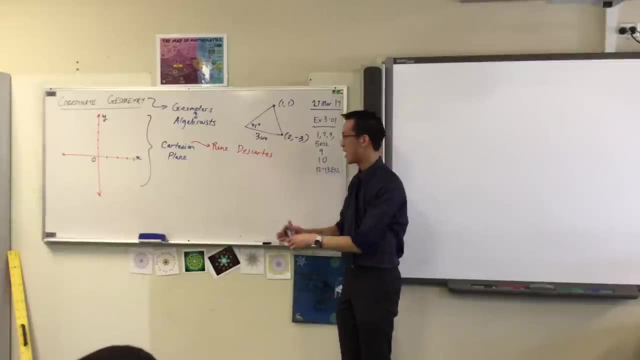 You usually only need a handful, okay. Secondly, not only is it very time consuming just to write 1, 2, 3, negative 1, negative 2, etc. It actually busies up your diagram and it becomes more and more. 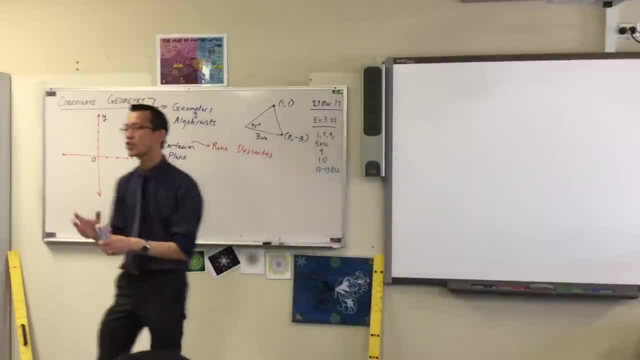 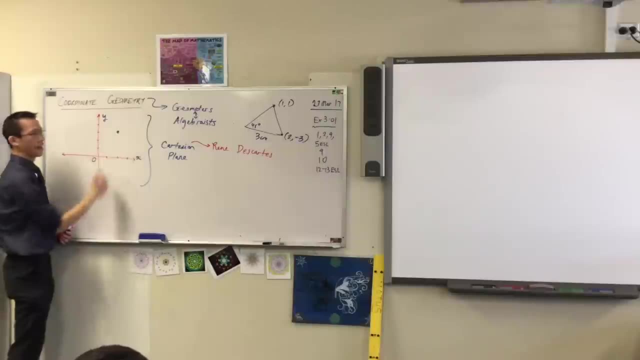 difficult to see. all the rest of the stuff which is more important, okay, So we're just going to label a few important bits. Let's pick a point. So, for instance, if I picked a point, say there, I'm going to draw that in. 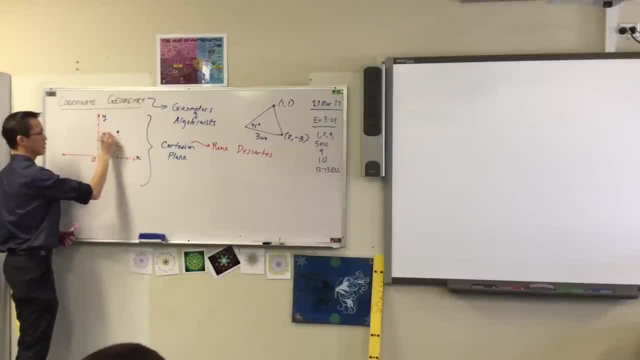 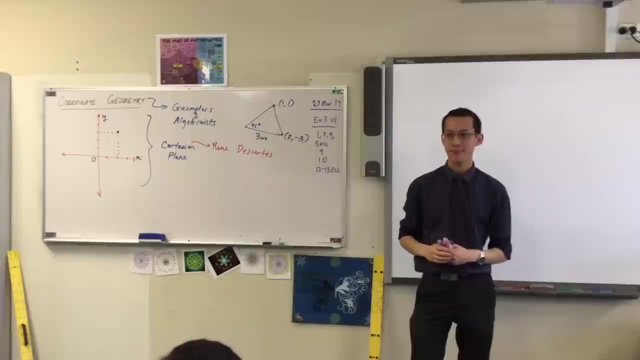 which is in line with this and this. So I'm going to raise the hand and describe. how would we describe the coordinates of that point? I drew up there. Any take? Yeah, Helen 2, 3.. Yeah, so I'm going to label this. 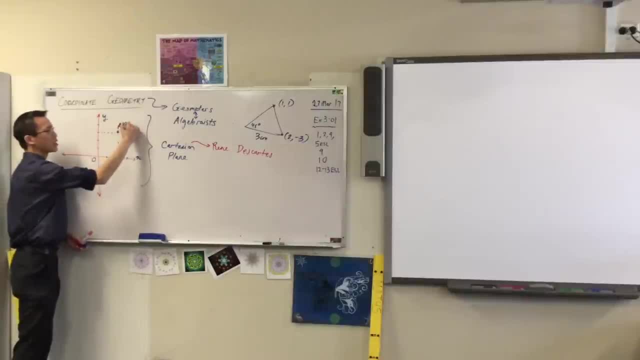 Let's actually give it a name as well. Let's call this guy A, And its coordinates do look like 2, 3 because, as you can see, you've gone across 2 units, then you've gone over 3.. 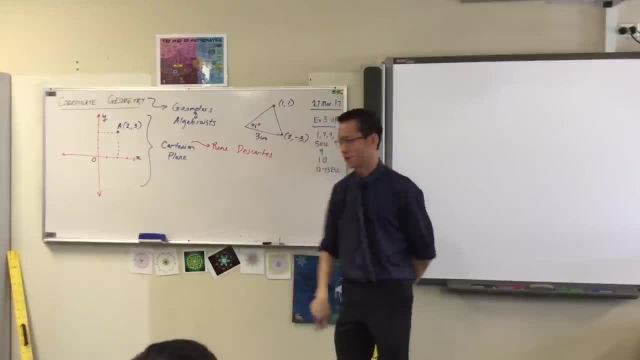 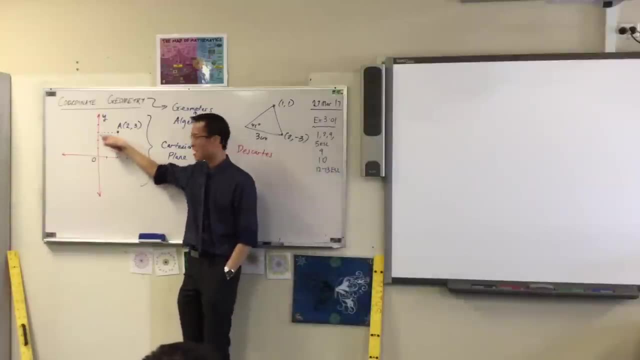 I will point out. I don't know if you started to draw numbers, because I was telling you not to, but I did not draw numbers, so that might not be 2, 3. It could be like 200, 300.. 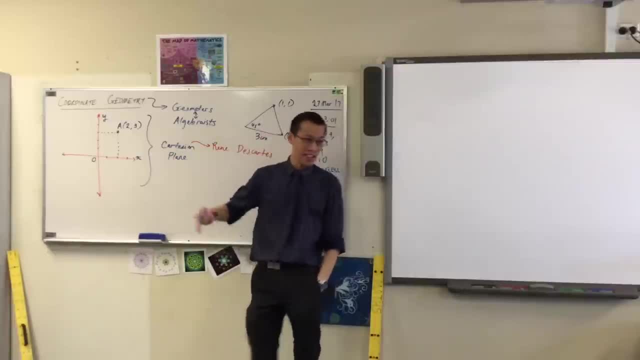 I don't have any sense of scale yet, but since we've called it 2,, 3, let's put a sense of scale on there. So now I'm going to mark in the 2 and the 3.. Okay, 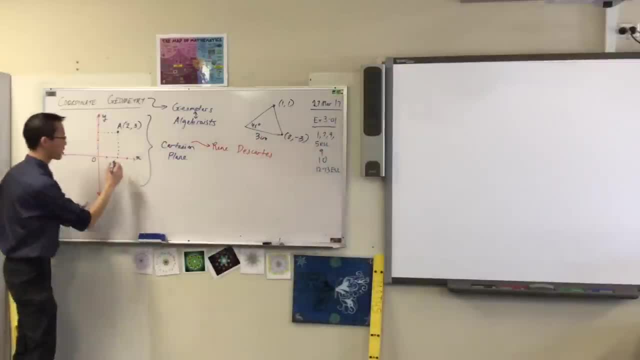 I don't have any sense of scale yet, But since we've called it 2,, 3, let's put a sense of scale on there. So now I'm going to mark in the 2 and the 3.. Now, on the side where you've written: 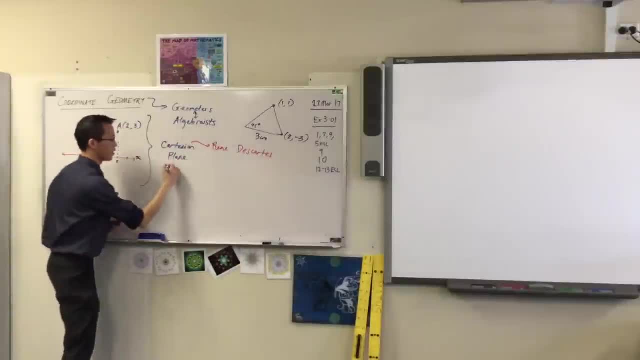 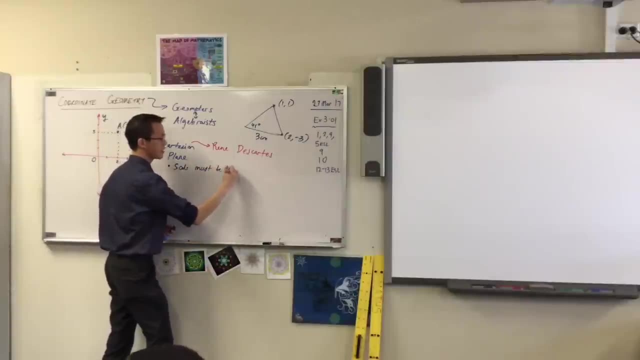 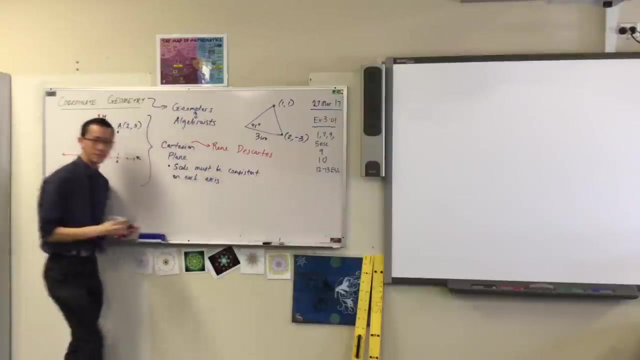 Cartesian plane. I want you to make two little subnotes. The first subnote is when you're looking at this scale. scale must be consistent on each axis. Let me explain what I mean. You see how we just said that's 2?. 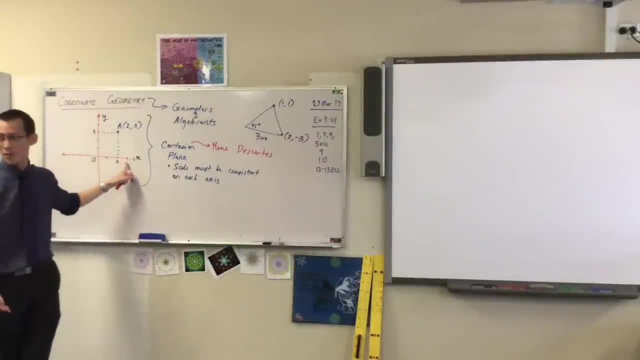 Well, if that's 2,, this next point being that it's equally spaced, it had better be 3.. Because look, that's the scale. If I then said I wanted a point like 10 comma 1, I can't say it's here. 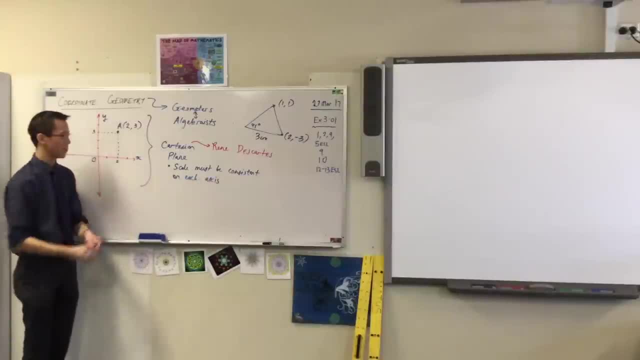 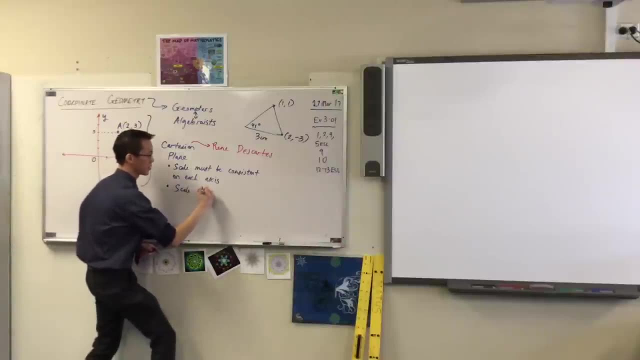 because then the scale would be inconsistent along each axis. However, while scale must be consistent on each axis, the scale can be different on separate axes. That's the plural for axis, by the way It's spelled, just the same way axis is. 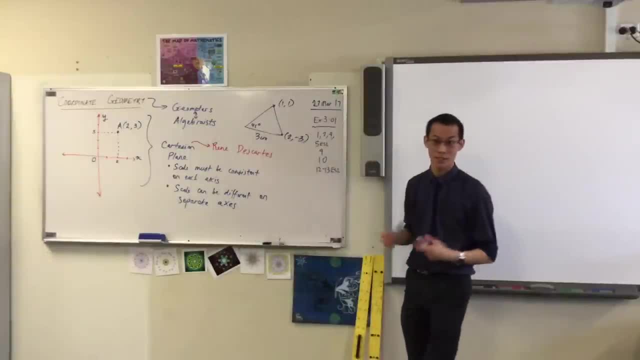 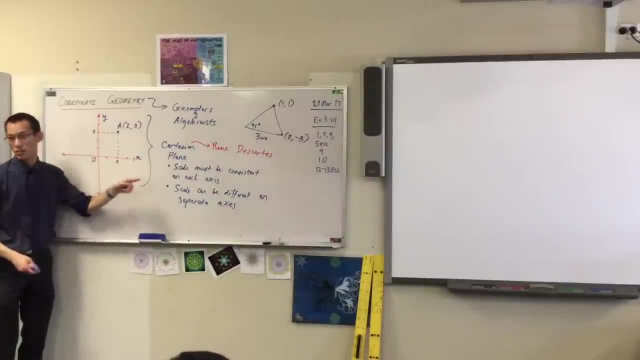 but we pronounce it axes, so you know we're talking about something different. So, for instance, just because I'm going one at a time along the x-axis, if I wanted to, I could still make this 2 comma 300, and make this 100,, 200,, 300.. 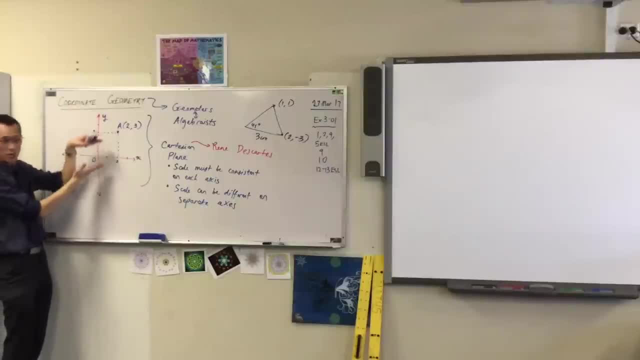 So long as it's consistent, on its own they can be different to each other. Does that make sense? Horizontal, vertical, they can be separate. In fact, sometimes they have to be really, really separate, because maybe this axis here might be about time. 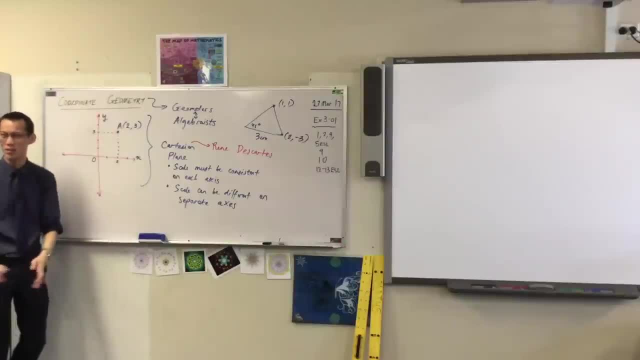 and this axis over here might be about temperature, So it's totally different units altogether. Alright, let's put another set of coordinates on here. Let's go to the left this time. So I'm going to label this point on the axis. 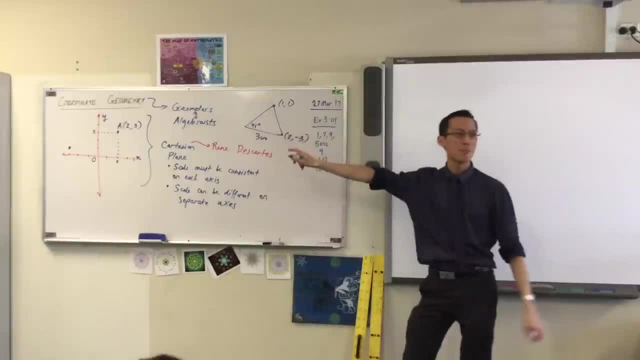 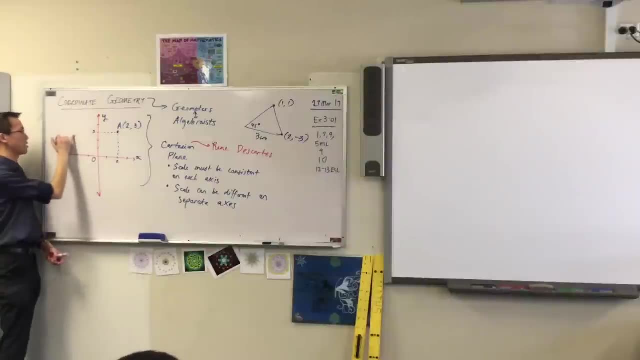 Now I've decided on a scale now, so hopefully you guys can tell me what would that point be. It's gone to the left, so I do my horizontal coordinates first. so this is, let's call it, capital B, shall we? 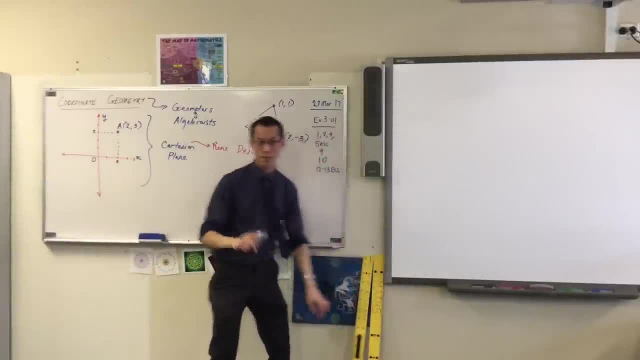 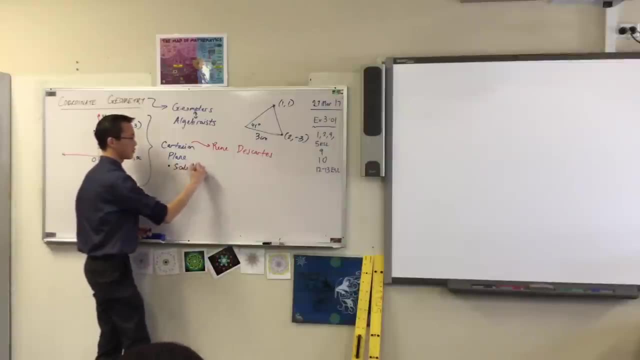 Now, on the side where you've written Cartesian plane, I want you to make two little subnotes, okay? The first subnote is when you're looking at this scale. right scale must be consistent on each axis. Let me explain what I mean. 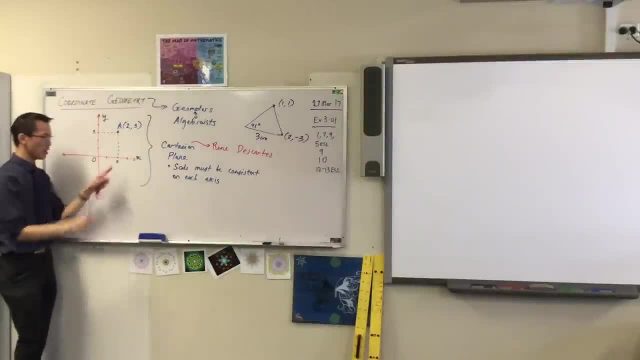 You see how we just said that's 2?. Well, if that's 2,, this next point being that it's equally spaced, it had better be 3, right, Because look, that's the scale. If I then said I wanted a point like 10, 1,. 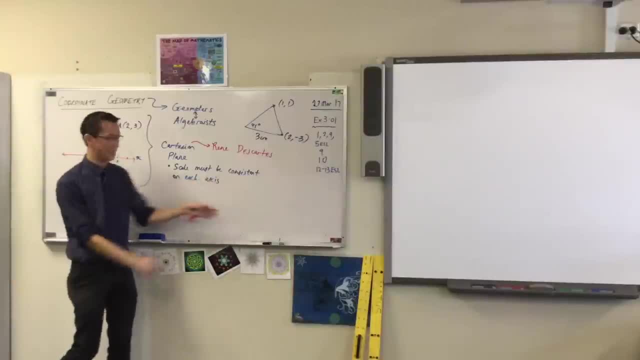 I can't say it's here, because then the scale would be inconsistent along each axis. okay, However, while scale must be consistent on each axis, the scale can be different on separate axes. That's the plural for axis, by the way. 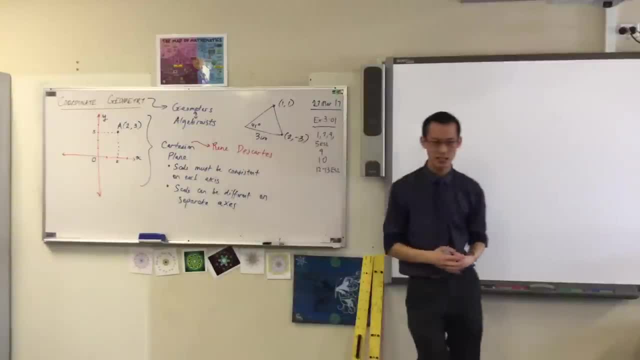 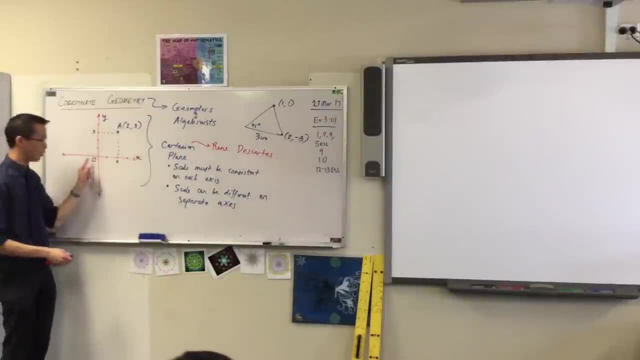 It's spelled just the same way axis is, but we pronounce it axes. we're talking about something different. So, for instance, just because I'm going one at a time along the x-axis- if I wanted to, I could still make this 2, 300. 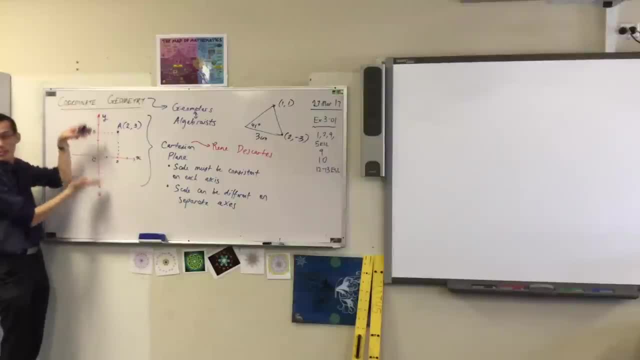 and make this 100, 200, 300.. So long as it's consistent, on its own they can be different to each other. Does that make sense? Horizontal, vertical, they can be separate. In fact, sometimes they have to be really, really separate. 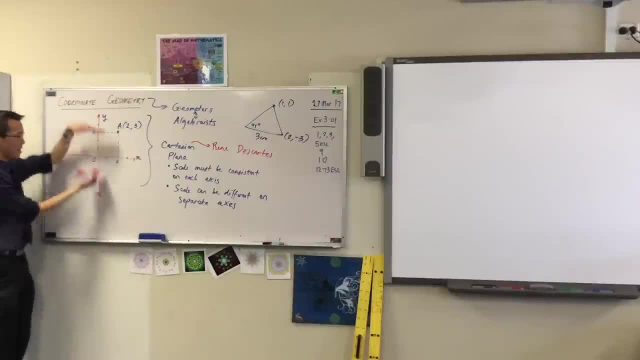 because maybe this axis here might be that time and this axis over here might be that temperature. So it's totally different units altogether. All right, let's put another set of coordinates on here. Let's go to the left this time. So I'm going to label this point on the axis. 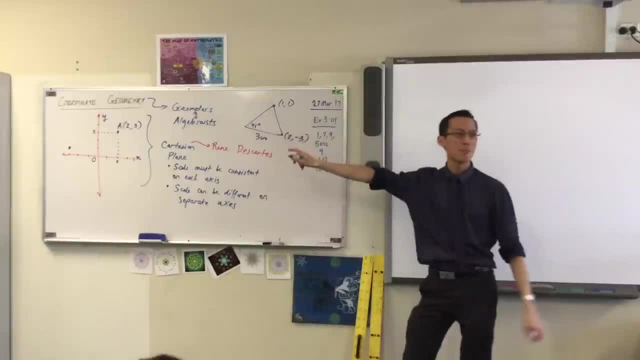 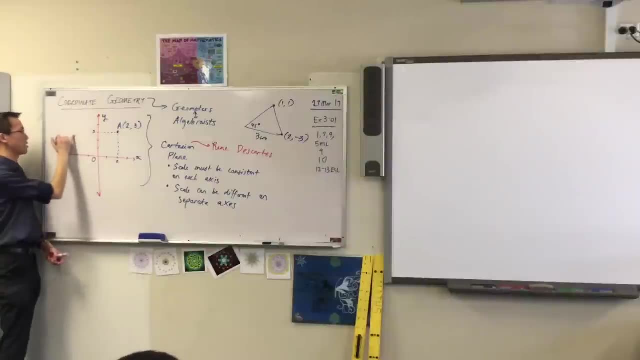 Now I've decided on a scale now, so hopefully you guys can tell me What would that point be? What would we call it? It's gone to the left, so I do my horizontal coordinates first. So this is, let's call it, capital B, shall we? 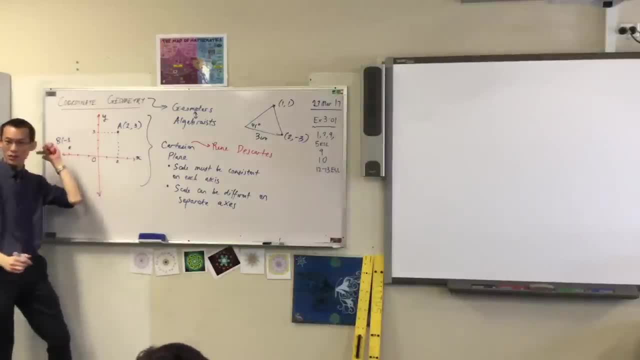 And it's negative. 3, I've gone that way to the left comma, what? 1.. Cool, So we do horizontal position first and I'll draw some dots so you can see it all there. Horizontal position first, and then we do vertical second right. 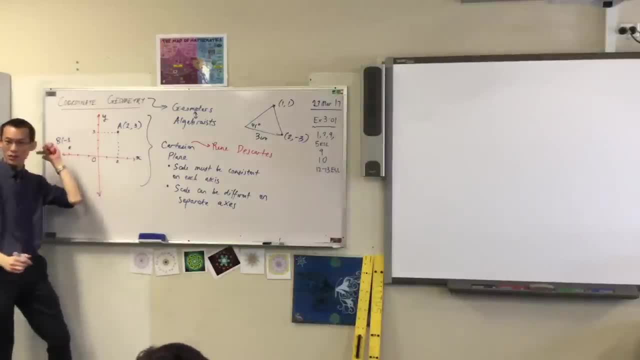 And it's negative 3, I've gone that way to the left comma: what? 1.. So we do horizontal position first and I'll draw some dots so you can see it all there. Horizontal position first, and then we do vertical second. 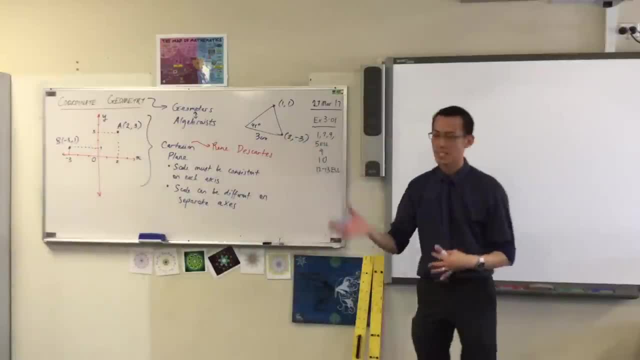 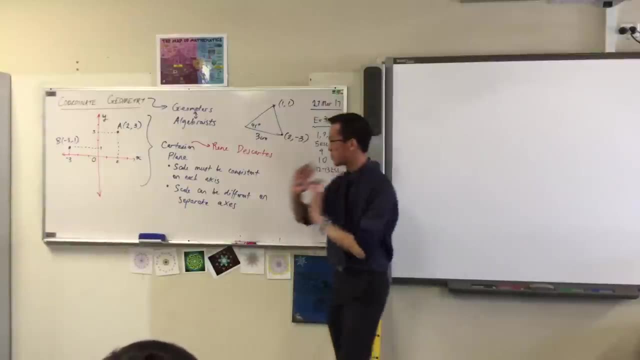 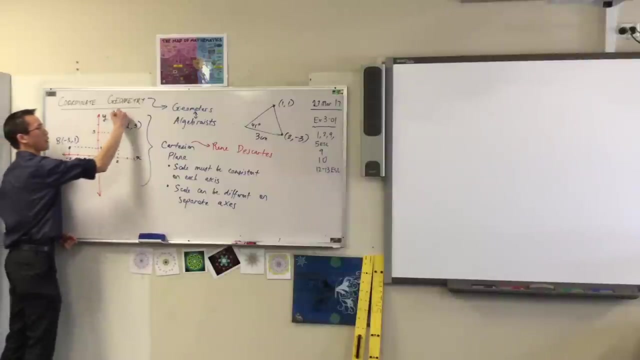 So it's alphabetical: Horizontal vertical x and then y. Okay, now, just really quickly, I will add on one last bit of notation onto here. You can see the Cartesian plane has been broken up into four regions. We give them names. 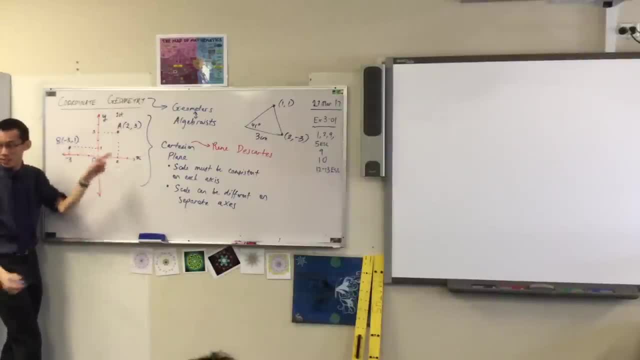 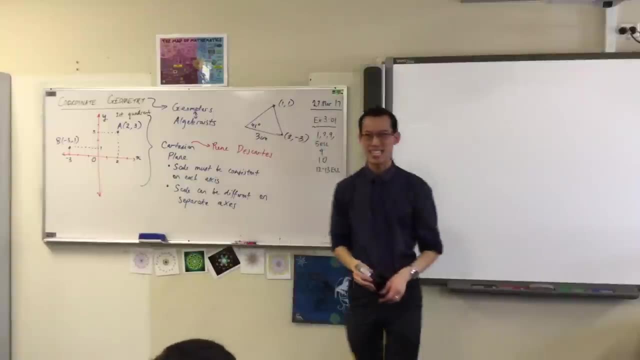 I've got another colour. it'll be helpful. We call this one over here, where everything is positive. we call it the first quadrant, Q-u-a-d-r-a-n-t Quadrant. Why do you think it's called a quadrant? 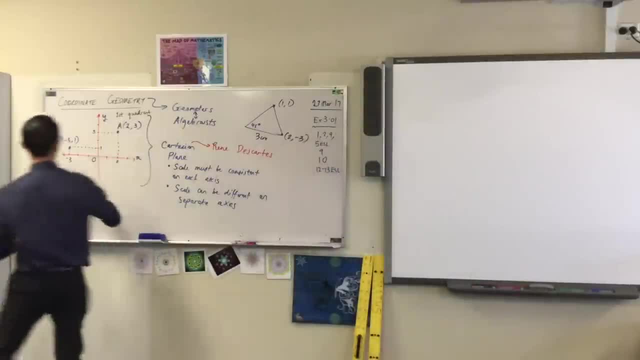 It's one out of four, right? So there's the first quadrant, you've got the second one. we go anticlockwise. second quadrant over here, then the third: your x values are negative and your y values are negative. 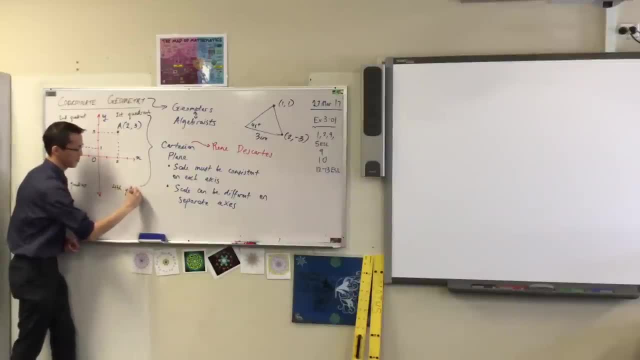 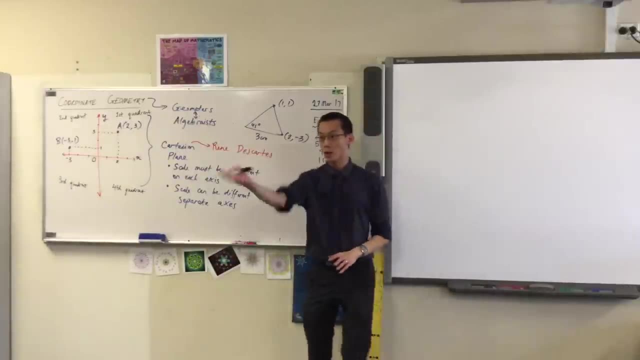 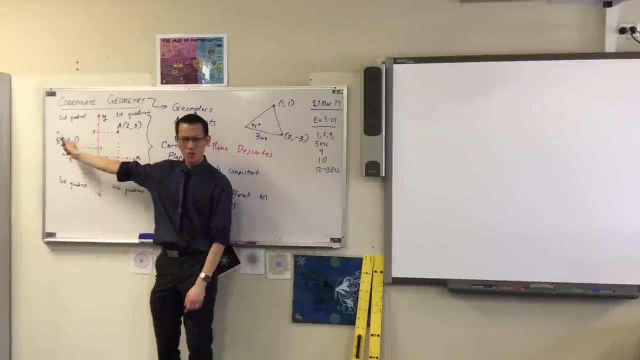 and then, lastly, the fourth. Okay, First, second, third, fourth. Now it's a great question as to- because I heard you didn't ask me, but you asked to the air. okay, Why is it that this is the first quadrant? 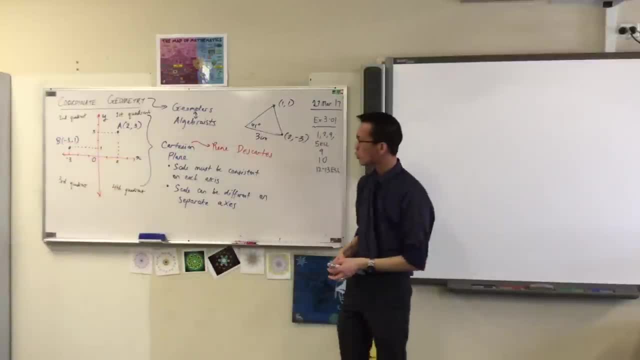 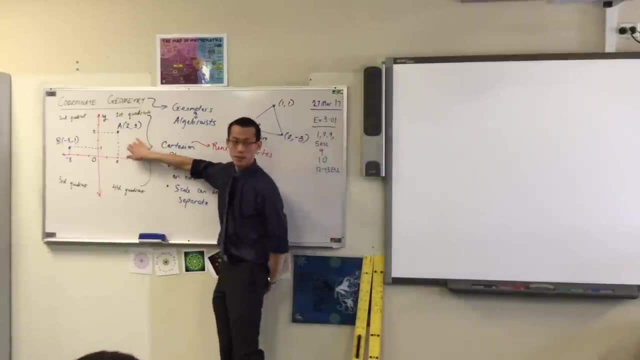 not this one. Like, that's a bit weird. in English we write from left to right, so why would we start over here? why, actually? there's a good reason why this is a good choice for the first quadrant. Alright, what do you think? 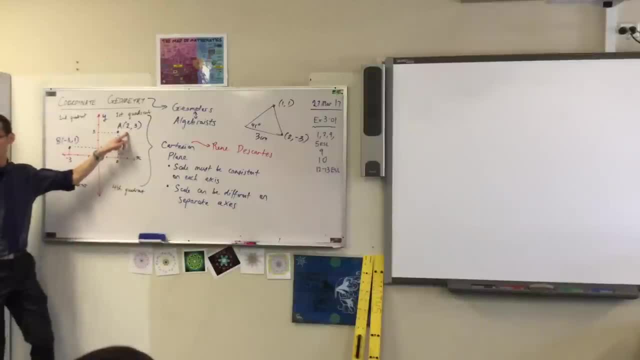 Okay. so the main thing is when you have a look at the values of the numbers, you're going to get all the positives over here, and we tend to start there because it's the easiest When you have a look at later on. 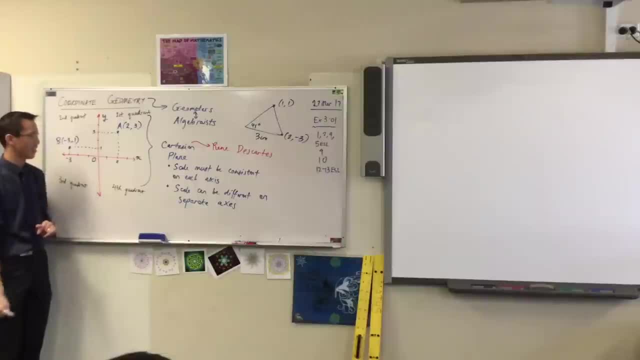 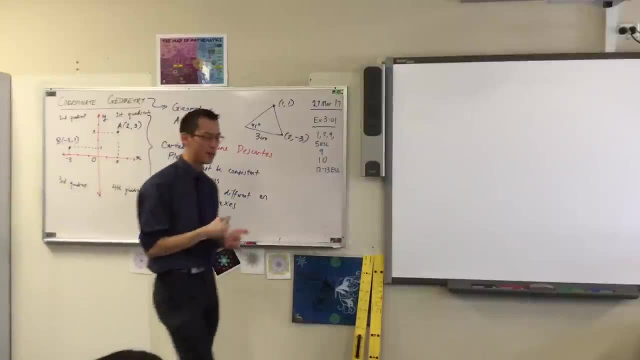 we're going to attach trigonometry to this. You did trigonometry last year. You thought it had to do with mainly triangles. I'm going to attach it to this as well. You will see, there's a really common sense reason why. 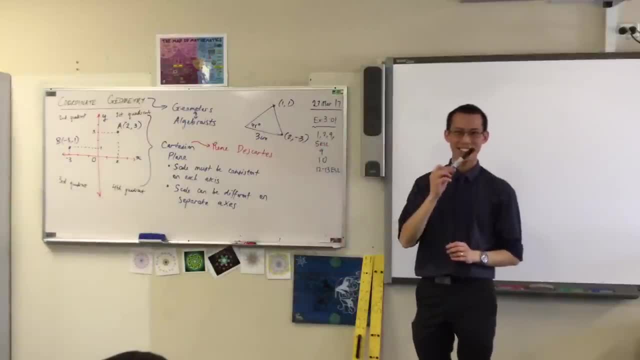 which is starting in the top right. even though for English doesn't maybe seem like it would make sense, mathematically it does make sense.